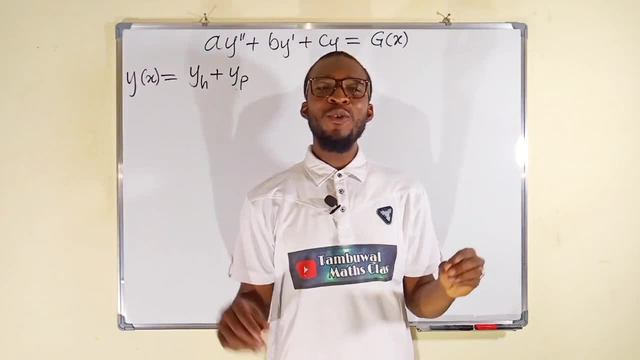 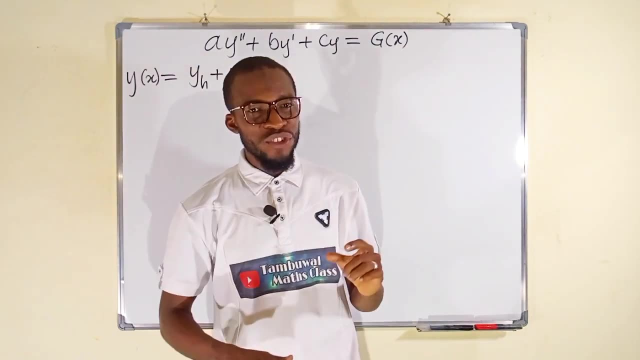 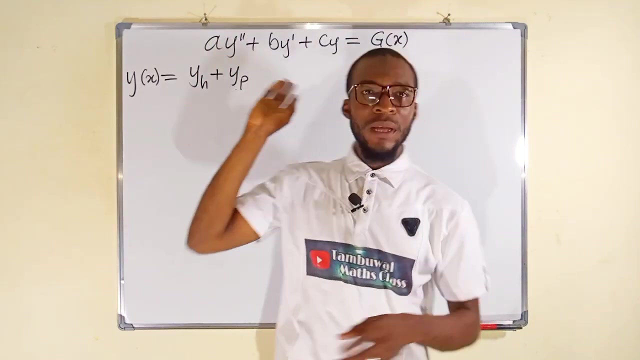 Hello, good day viewers. In this tutorial, I am only going to guide you through the various steps required in order to find the solution to second order linear, non-homogeneous differential equations by the method of undetermined coefficients. So we have the general form. here You can see the general form of second order linear, non-homogeneous differential equations. 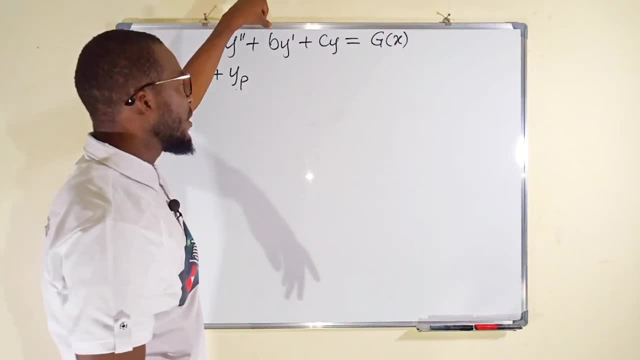 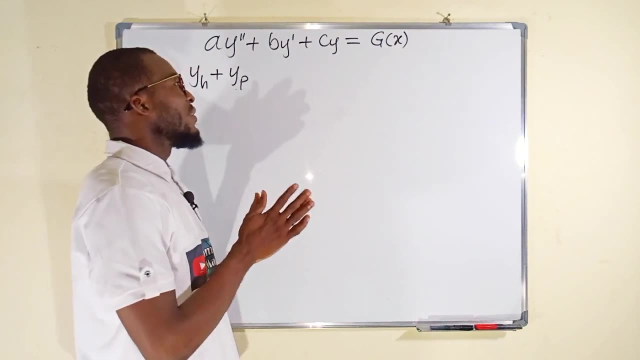 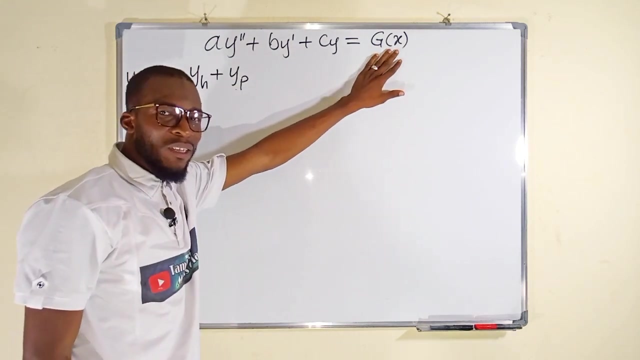 We have a, y double prime plus b, y prime plus cy, equal to g of x, where a, b and c are all constants. So what differentiates this from the homogeneous type? in homogeneous differential equations, The g of x is said to be equal to zero. talking about second order linear, 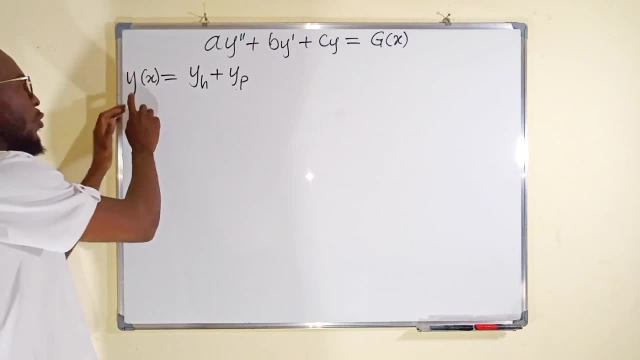 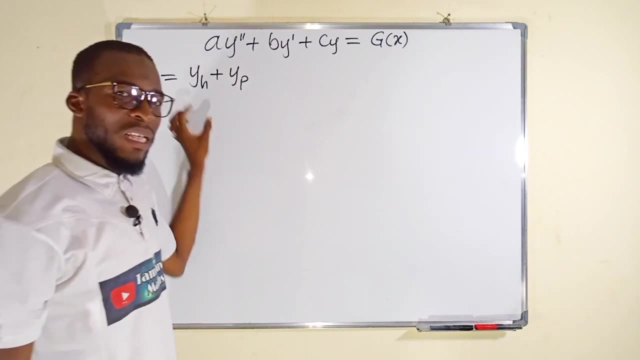 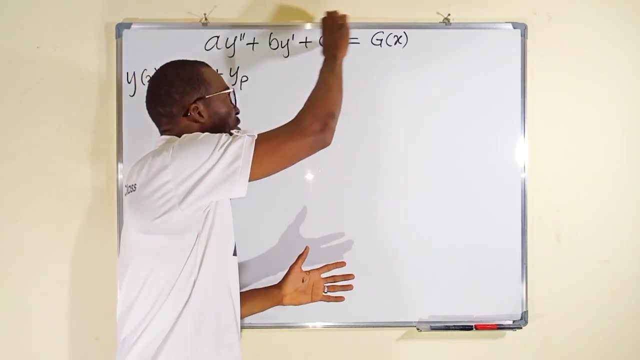 So to find the general solution to this problem, we are going to take y, which is a function of x equal to y sub h, plus y sub p. This y sub h is the general solution to the homogeneous differential equation. This means that we are going to set the whole of this equation to be equal to zero, setting g of x to be equal to zero. 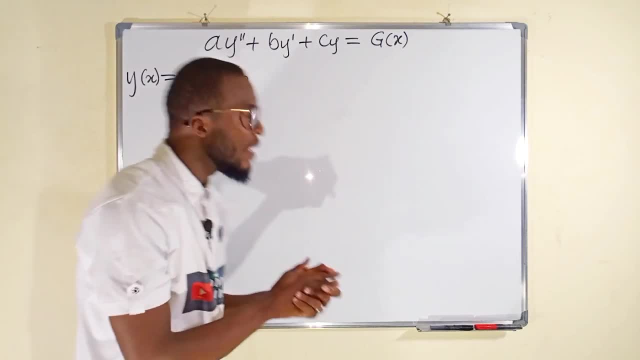 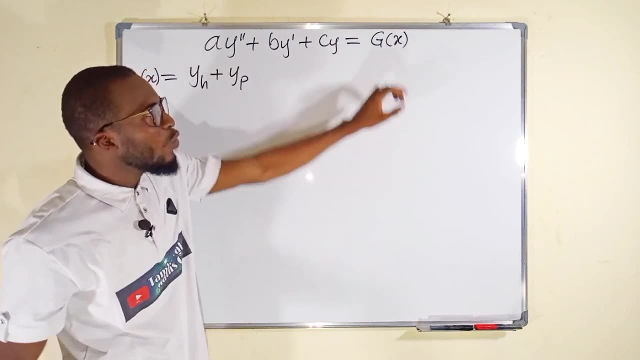 Solve for the homogeneous type and keep the result aside. Then you come for the particular solution, And particular solution could be obtained based on the nature of g of x. So I am going to guide you through the various steps required to find the solution. 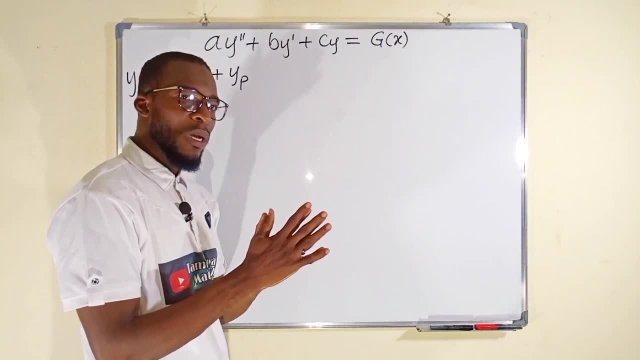 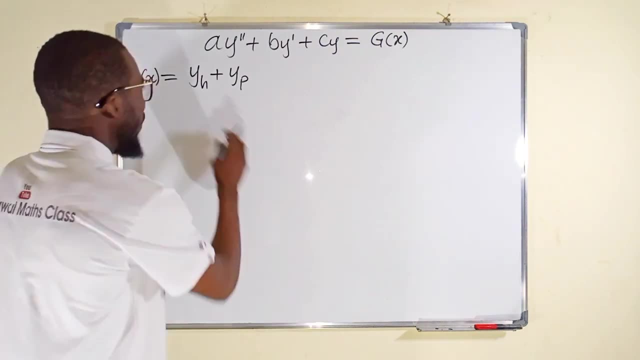 Y sub h and y sub p, because adding the two is said to be the general solution to the problem. Okay, let me start with y sub h To find the solution to the homogeneous type. you are going to set the whole of this equation to be equal to zero. 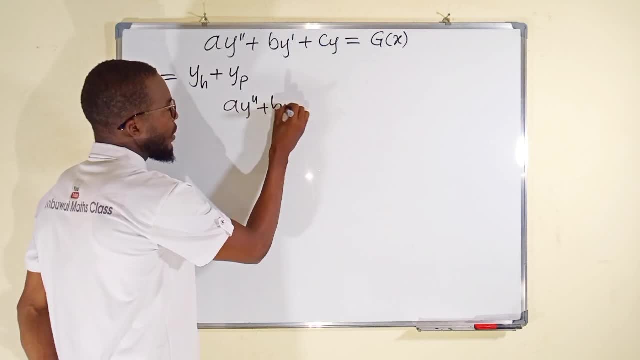 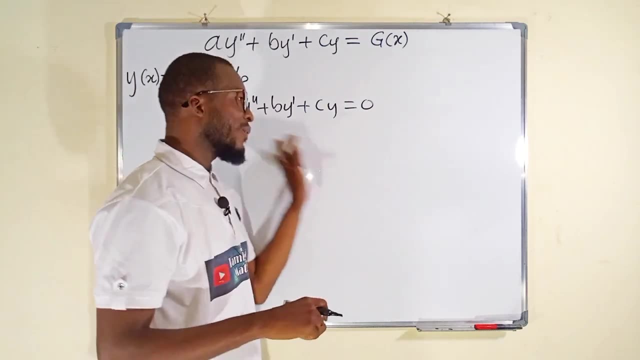 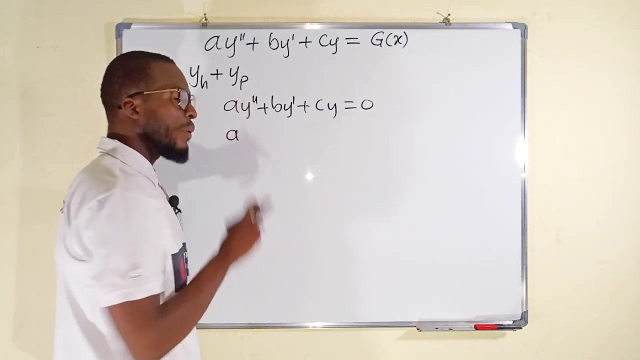 We have a y double prime plus b y prime plus cy equal to zero. Next we are going to transform the equation into an auxiliary equation. A constant y double prime should be replaced with r to the power of two or r squared. 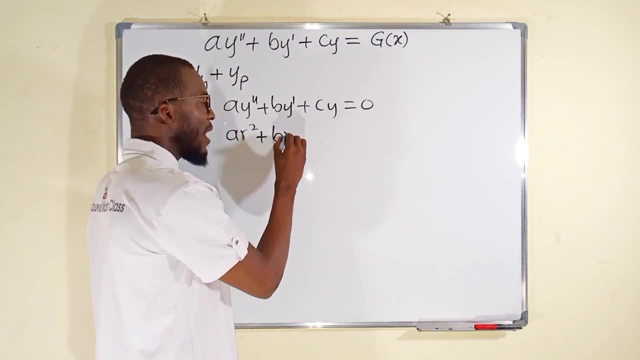 Plus b instead of y prime, we have r to the power of one. You can see the power is reducing by one. And lastly, we have c, because r is now to the power of zero, which is equal to one, equal to zero. 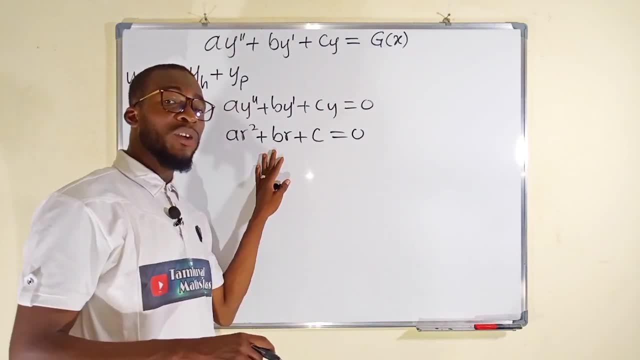 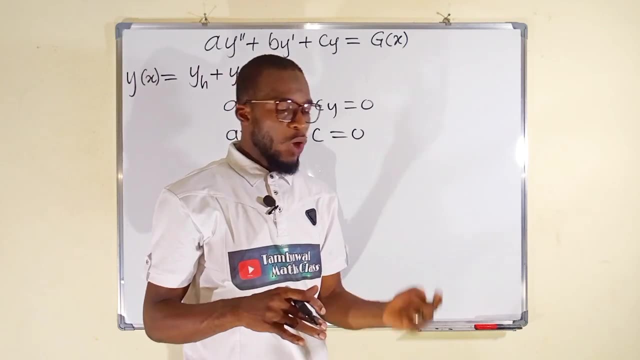 You can see this equation is now quadratic, which we have to solve for the roots. Therefore, the general solution to the homogeneous type depends on the nature of the roots. You have three forms of roots: real and distinct. real and equal and complex solution. 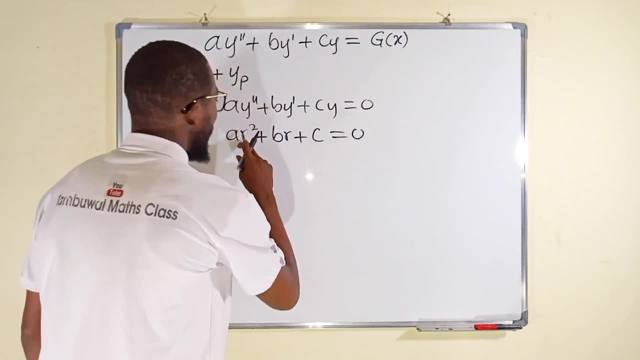 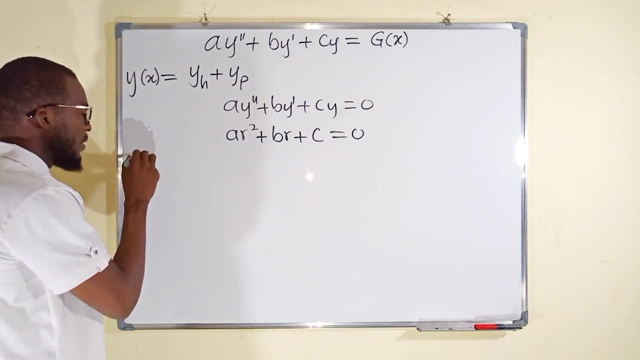 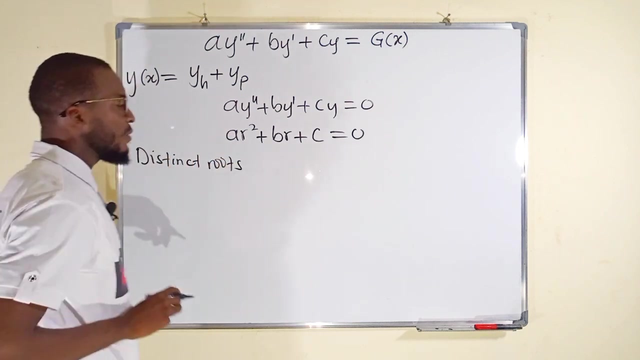 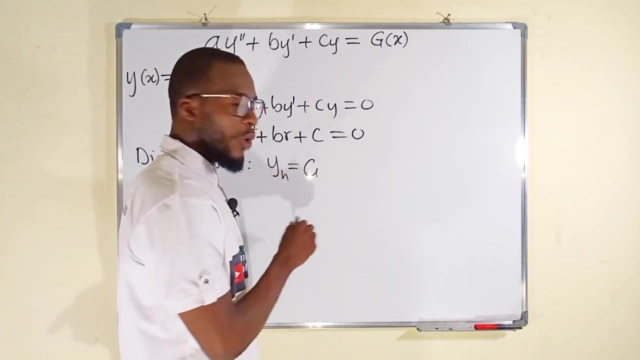 So suppose, after solving this, you realize the values of r are real and distinct, having two different solutions, Distinct roots. If you obtain real and distinct roots, the general solution to the homogeneous type will be a constant. let's call it c1,. 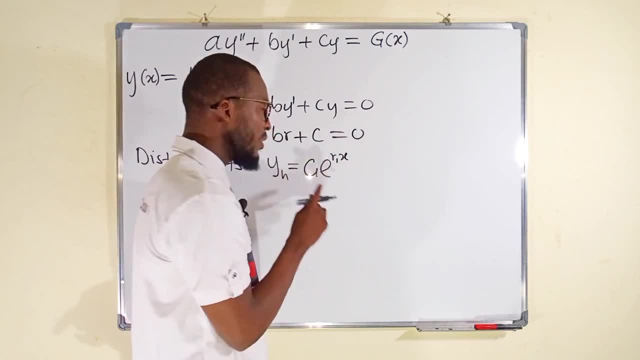 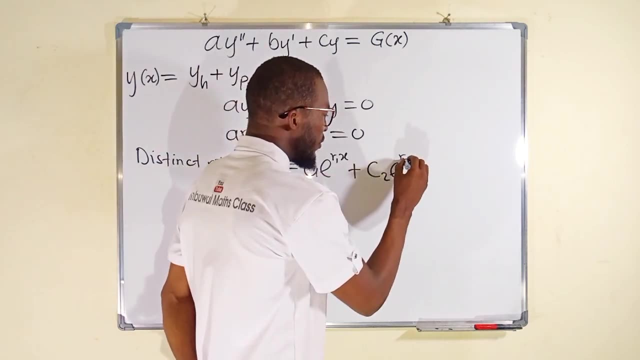 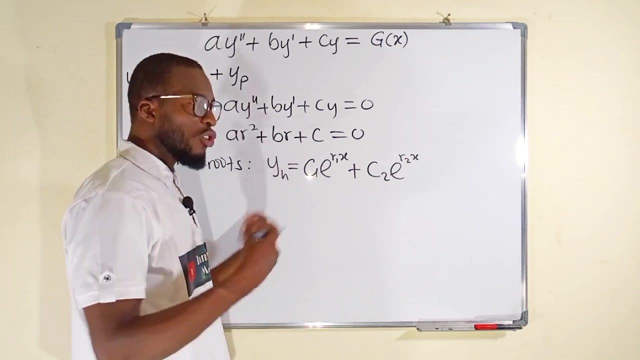 multiplied by e to the first root multiplied by x. So let's let that root be r1, plus another constant, c2, e to the second root multiplied by x. So this is going to be the general solution, But sometimes solving this quadratic equation may result to real and equal roots. 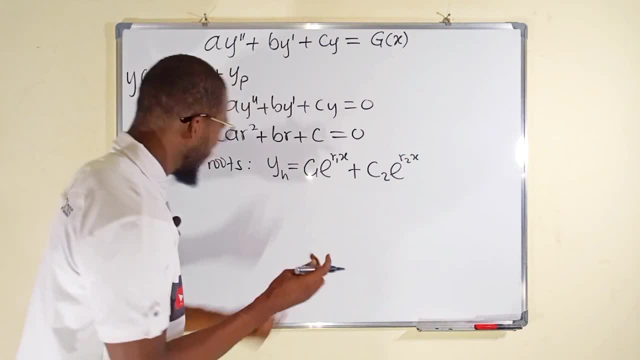 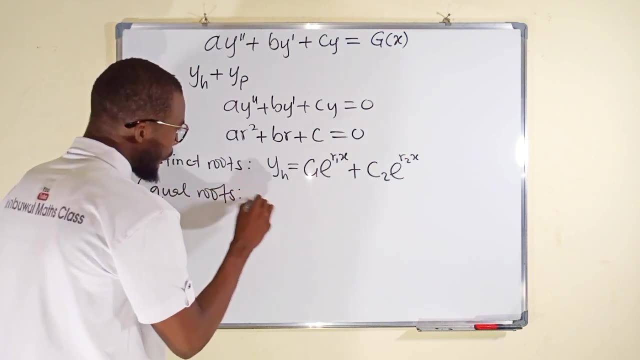 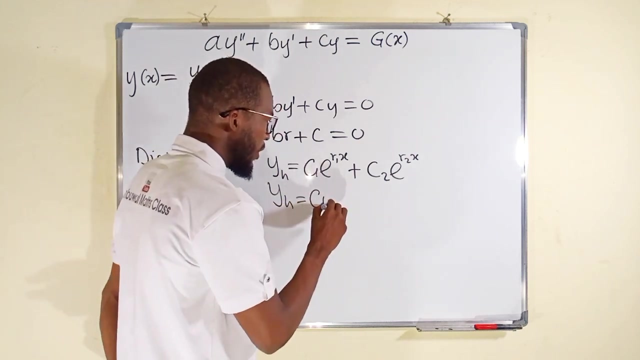 having two solutions of the same kind. So for real and distinct roots. so for real and equal roots. we have the general solution to be equal to a constant. let's call it c1, e to the rx. we don't have to write r1 and r2 because all the roots are the same. 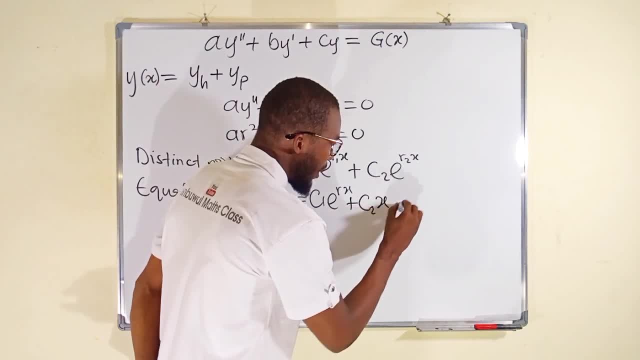 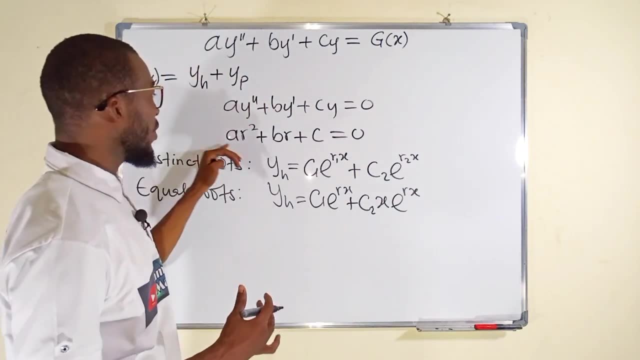 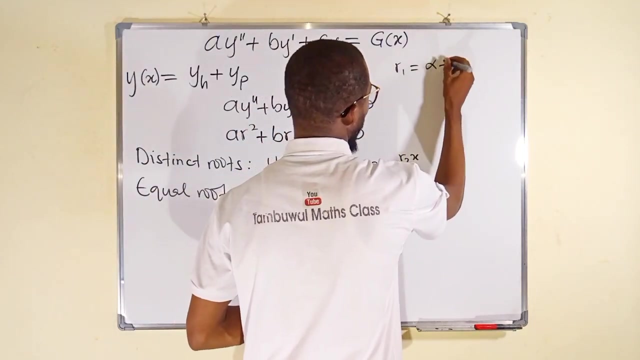 plus c2,, but this time around multiplied by x, e to the rx. So for real and equal roots, this is the general solution, But sometimes solving the quadratic equation may result to a complex solution, For instance if the first root is equal to alpha plus beta i. 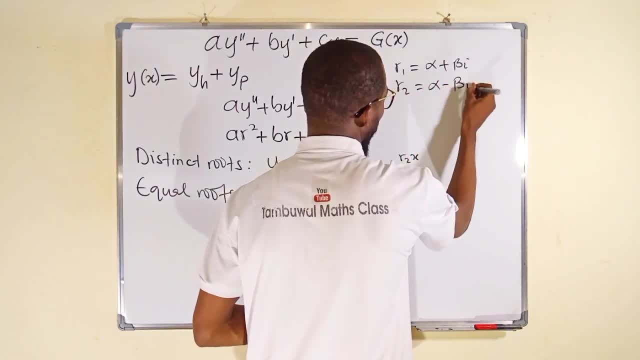 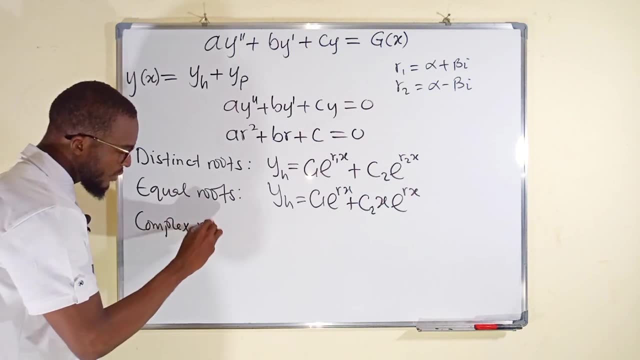 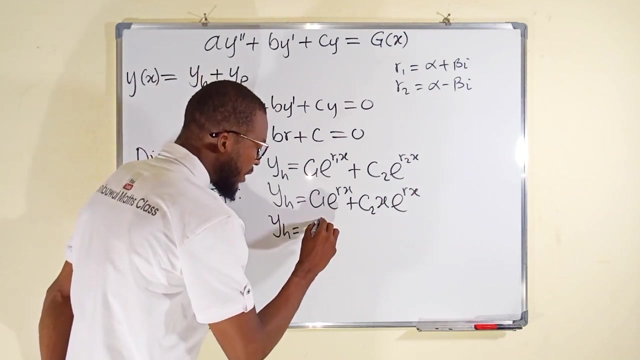 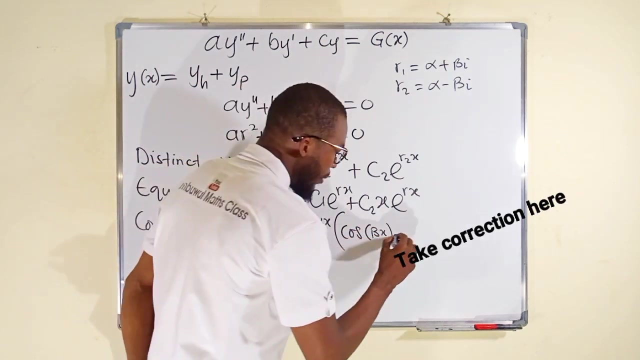 and the second one equal to alpha minus beta i, the general solution will be different. So for complex roots we have the general solution to be equal to e to the alpha x. then you multiply by cos of beta x plus sin of beta x. 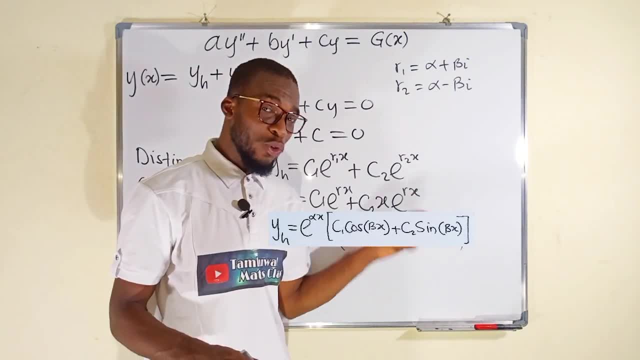 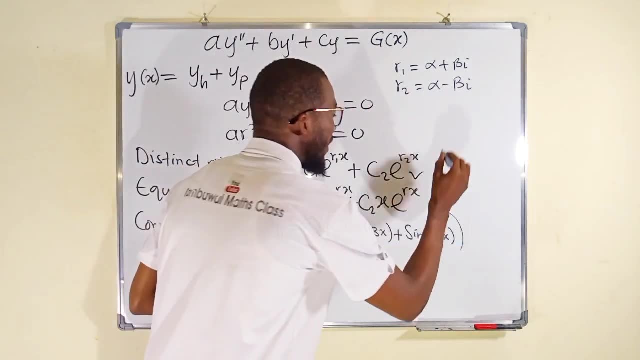 So for complex root, this is going to be the general solution to the homogeneous differential equation, talking about second order linear. But let us just assume that this is what we have of 10.. Because I told you I'm not going to solve any problem. 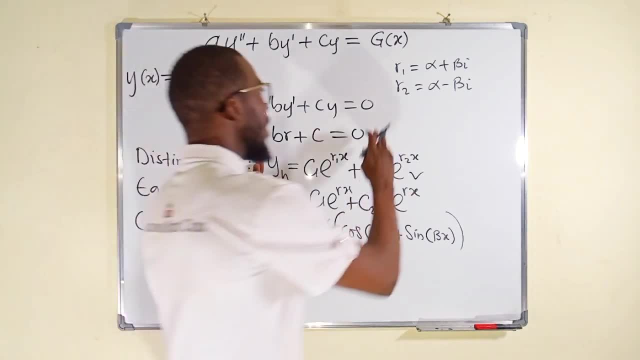 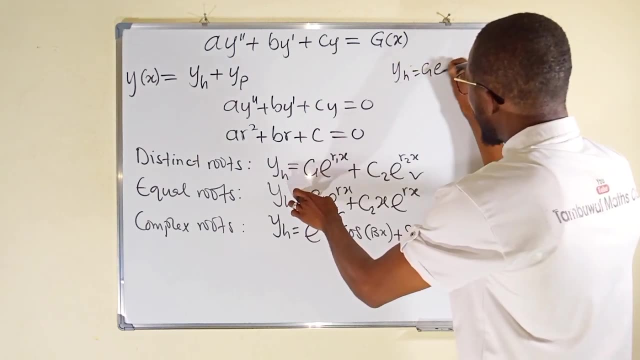 I'd rather take you through the various steps. So first, this is what we have. I'm going to keep it aside and go for the particular solution: y of h, equal to c1 e to the r1 x plus c2 e to the r2 x. 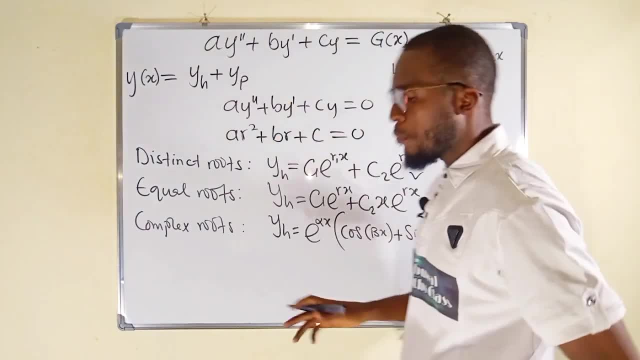 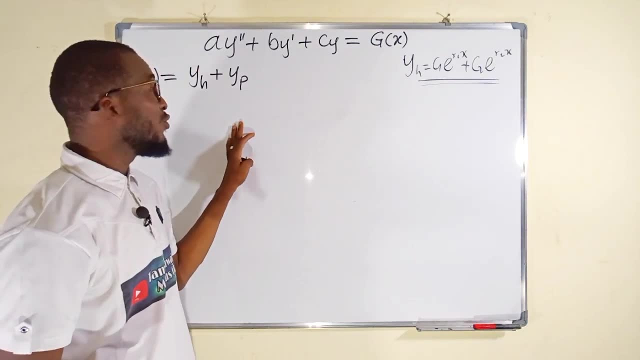 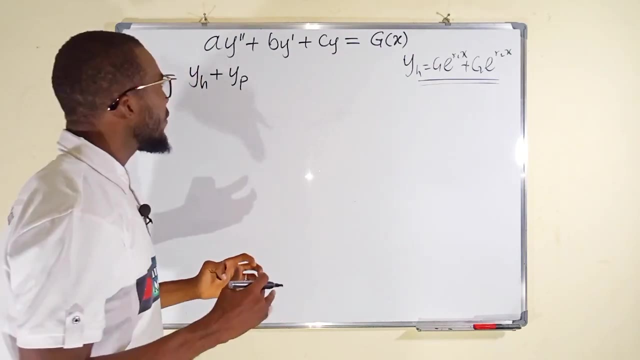 So now, let me wipe all this and go for the particular solution. So to find a particular solution, remember I told you that solution depends on the nature of g of x. We want to come up with a function which, if you take the second derivative, 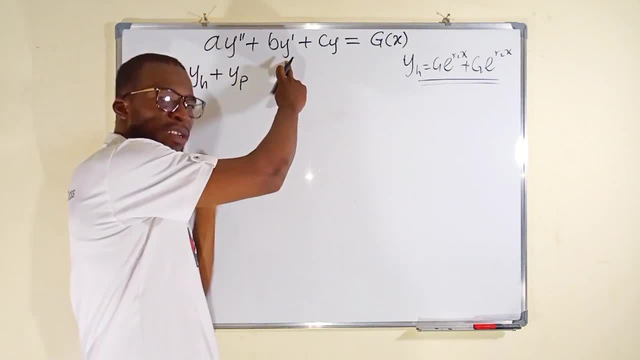 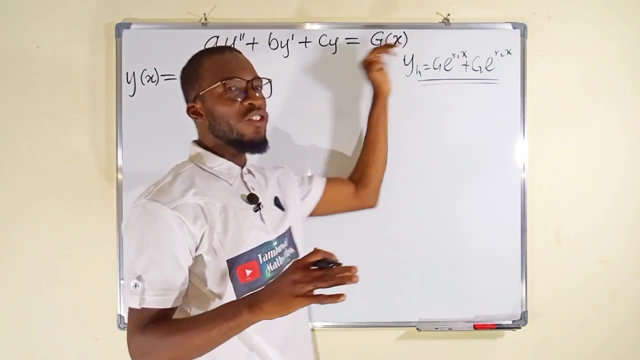 of that function, multiply by a first derivative of that function, multiply by b plus the function itself, multiply by c, it will be exactly equal to g of x to the right hand side. And how can we come up with this function? 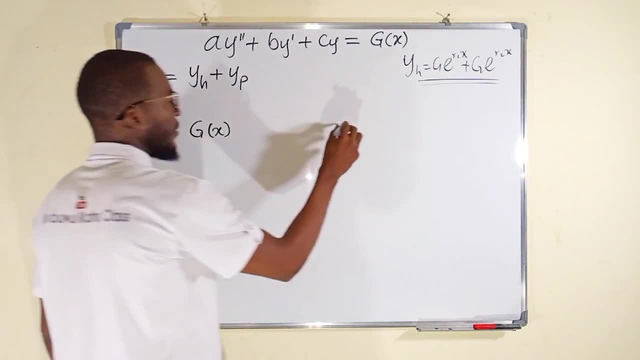 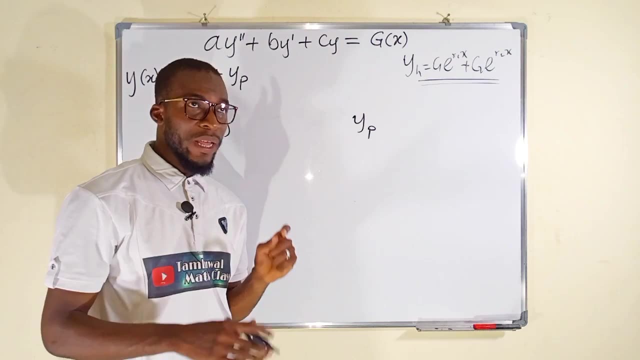 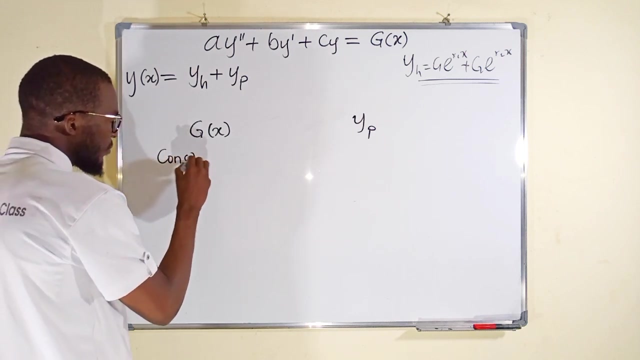 So let me write g of x here and y sub p here, If g of x is any constant apart from 0, like 2,, 3, minus 1, minus 10, and so on, If it is a constant. 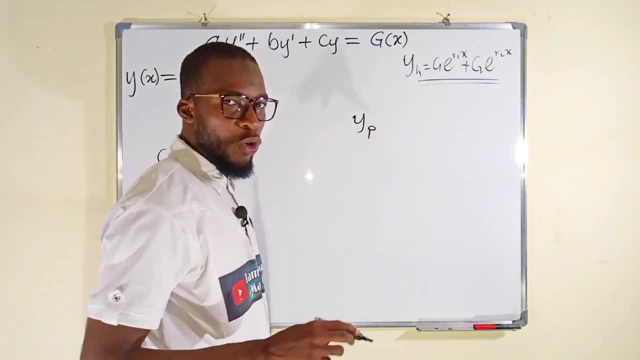 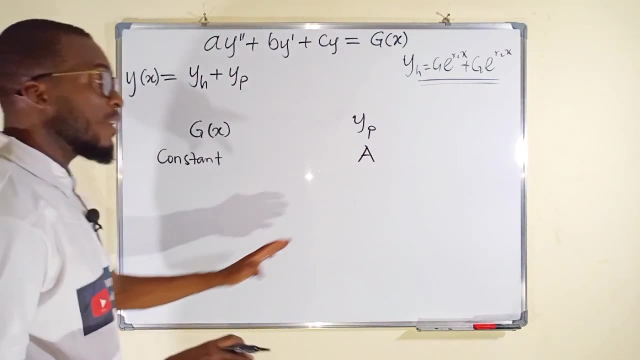 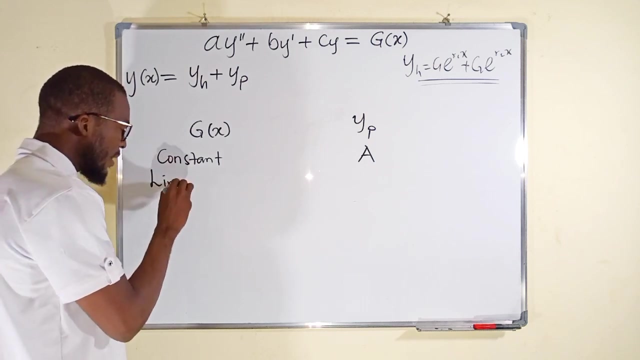 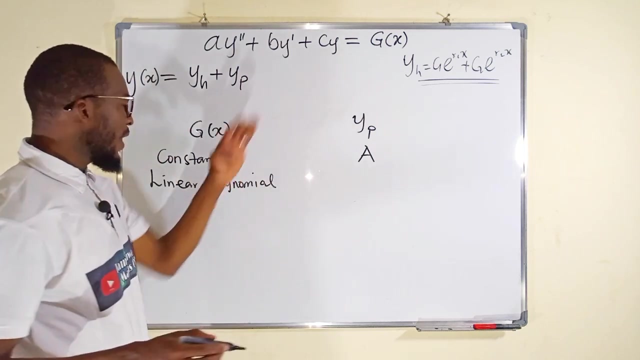 just take y sub p and equate it to be equal to a constant a or b or any letter, any constant. then in the end you are going to solve for that a If it is a linear polynomial, linear if g of x is a linear polynomial. 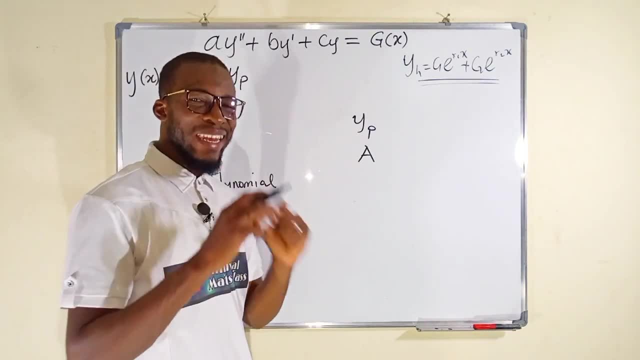 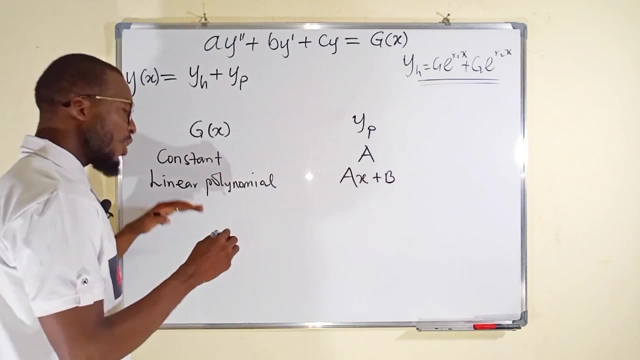 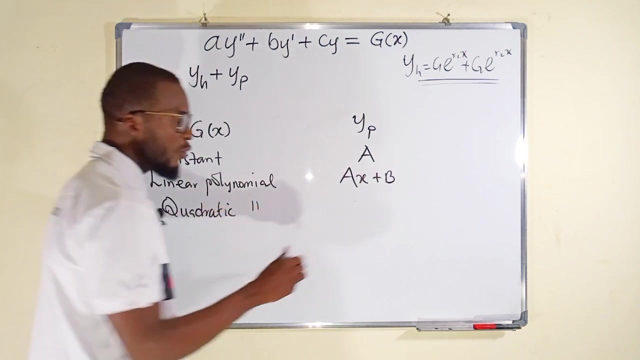 we are going to replace y sub p with a linear polynomial And the general formula you know it is ax plus b. If it is quadratic, let me add one more quadratic, quadratic polynomial and we are going to set y sub p to be: 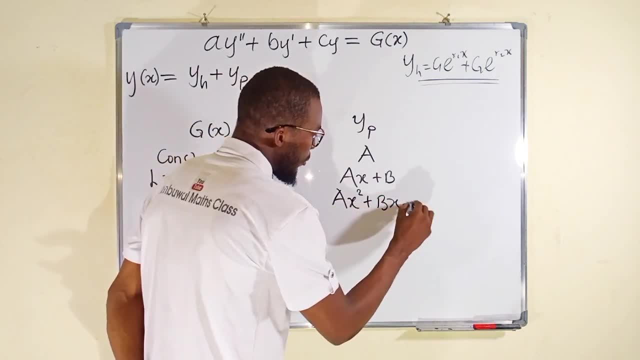 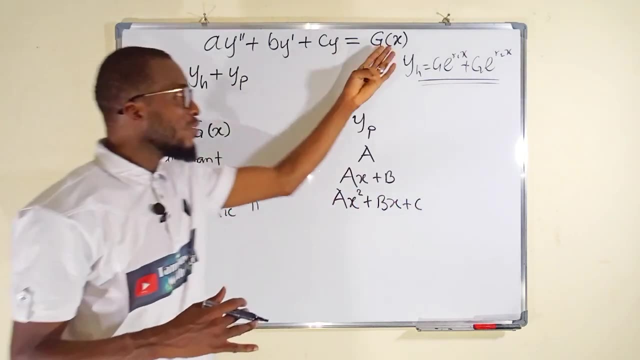 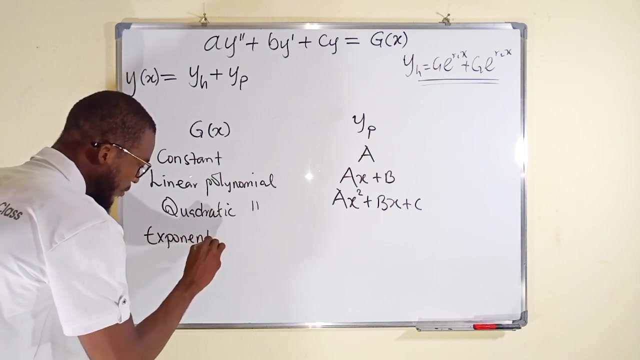 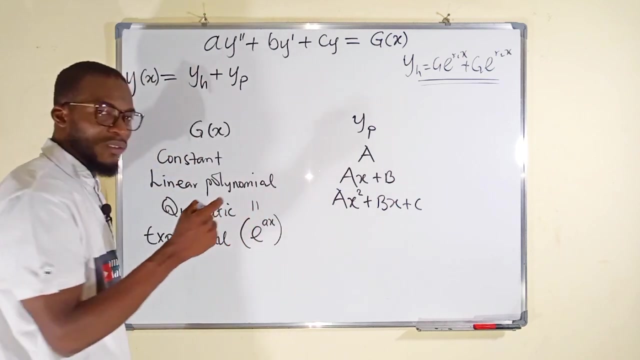 ax to the power of 2, plus bx plus c. You know this is general form of a quadratic function. So what if the function is an exponential function, Exponential. If it is exponential function, like exponential ax, where a is constant. 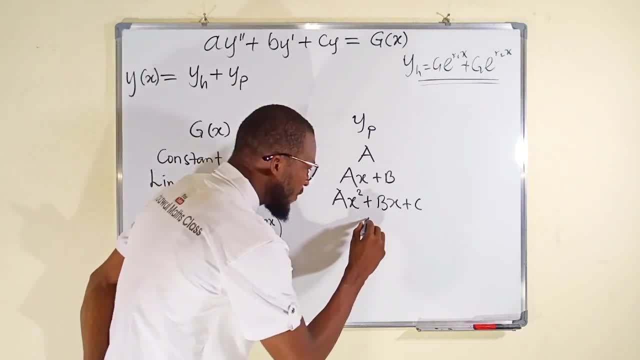 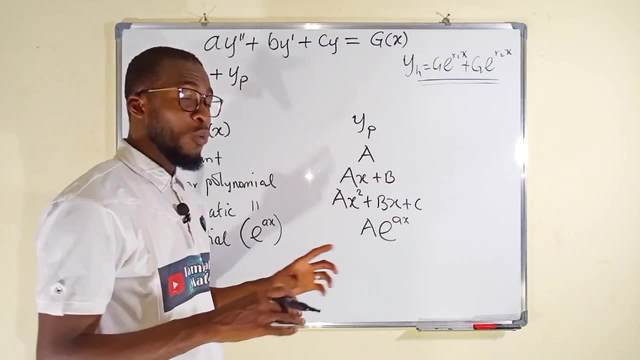 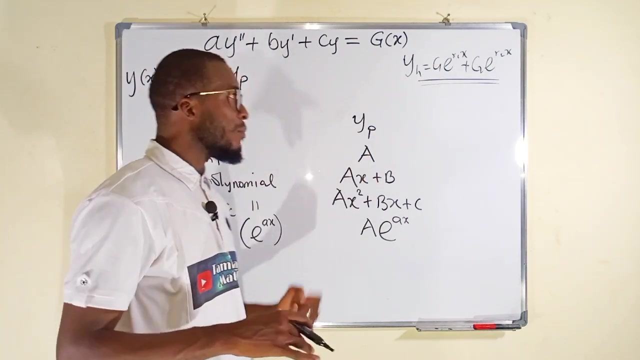 you are going to replace y sub p with a constant multiplied by e to the ax. The letter solves for this a. You know we are talking about undetermined coefficients, So these coefficients are said to be undetermined. In the end we have to find them and replace back. 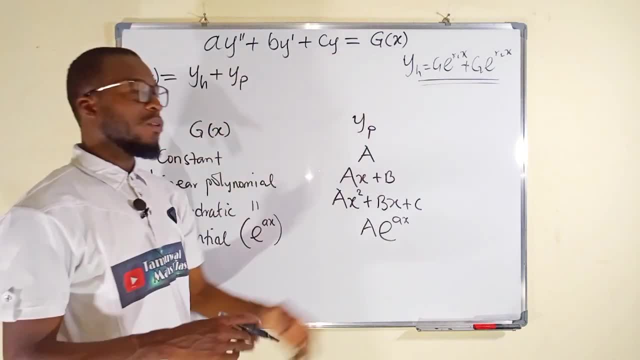 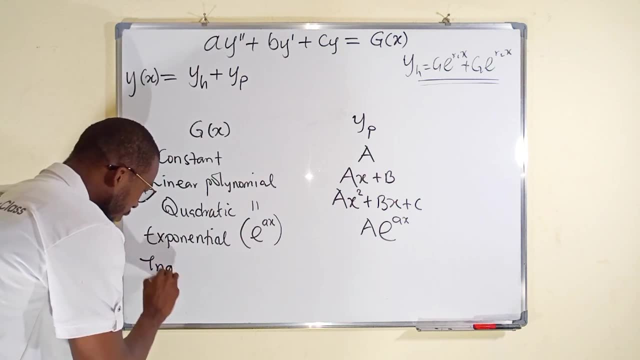 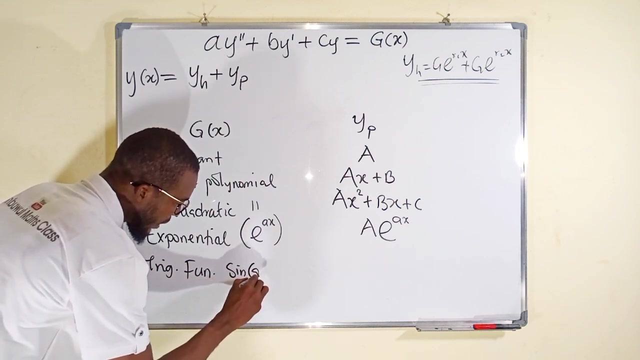 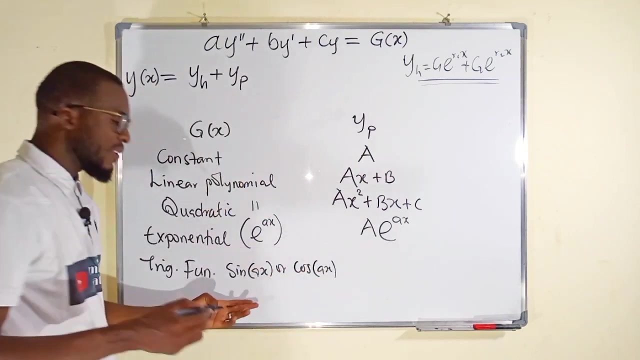 So sometimes this function g of s could be trigonometric function, like- let me write it here- trig, trig function like maybe sine ax or cos ax. All of these are said to be trigonometric functions. We are going to replace y sub p. 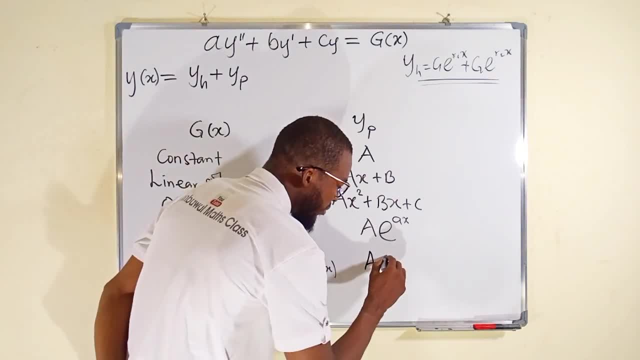 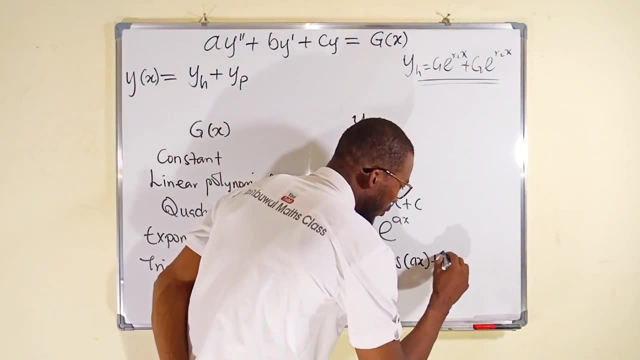 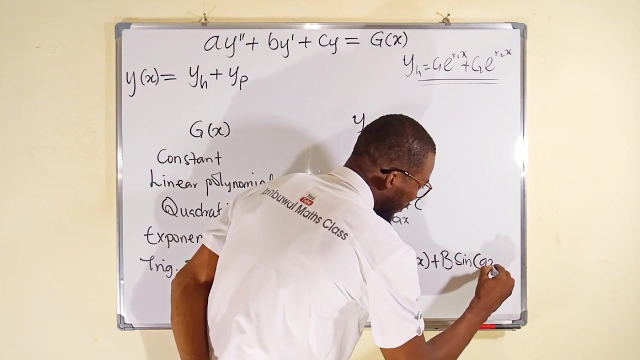 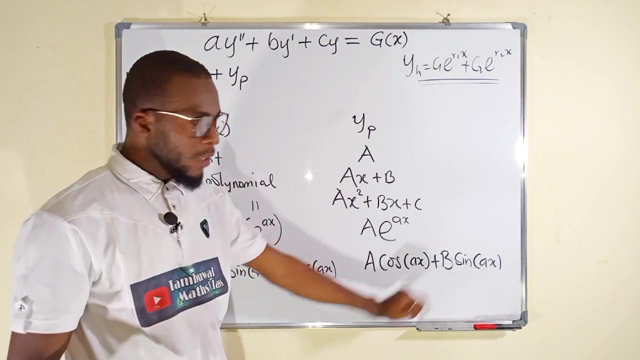 with a constant multiplied by cos of ax. Then you add another constant, b, multiplied by sine of ax. So if it is trigonometric function like this one, you should replace y sub p with this. So let's assume what we have as g of x. 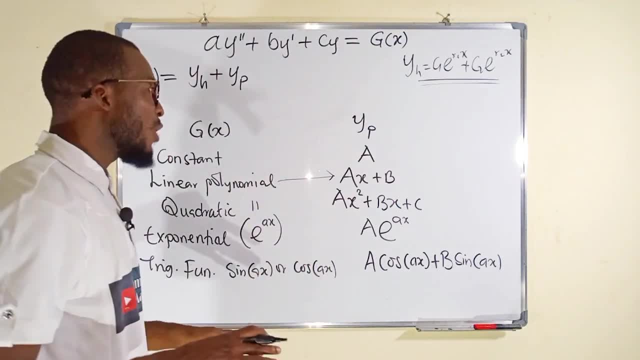 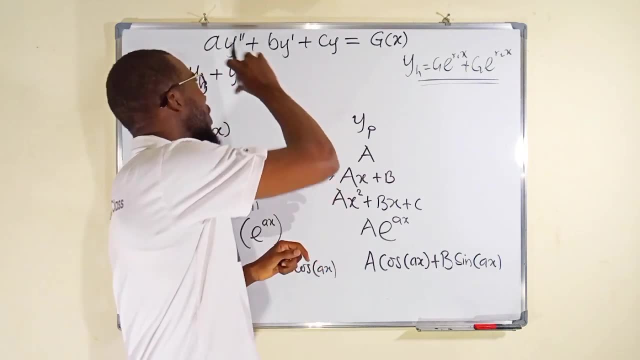 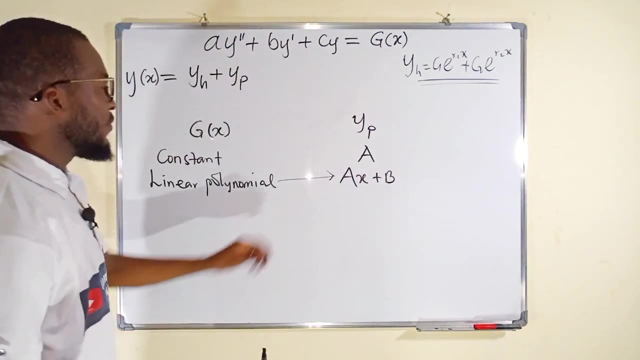 is linear polynomial. If it is linear polynomial, we are going to consider y sub p, with ax plus b. So let us use this one as an example to show you how we can find the general solution to the entire equation. So if g of x is a linear polynomial, 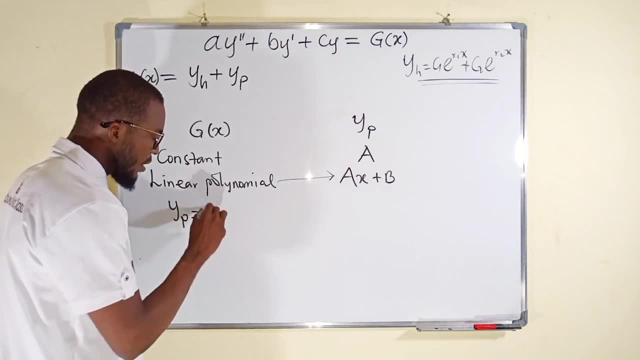 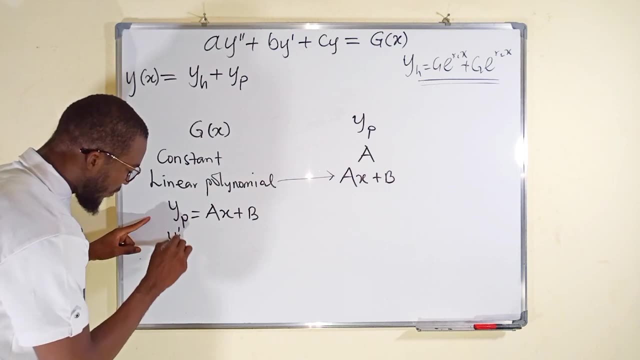 we are going to take y sub p and equate it to be equal to ax plus b. What do we do next? We find the first derivative of this function. You know we are going to differentiate with respect to x. If you differentiate this, 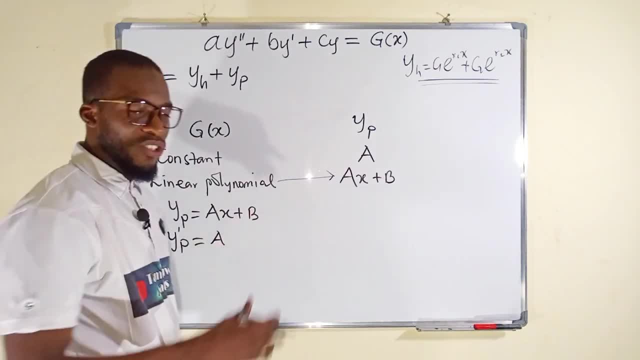 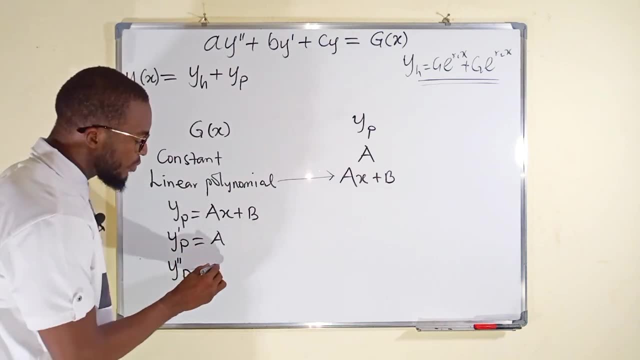 x will go live in a, and this is constant. If you differentiate it you get zero. You have to find the second derivative as well. You know second derivative is going to be zero because derivative of constant is zero. So we are going to replace. 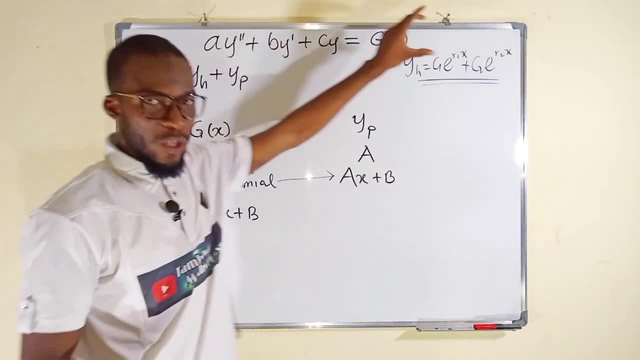 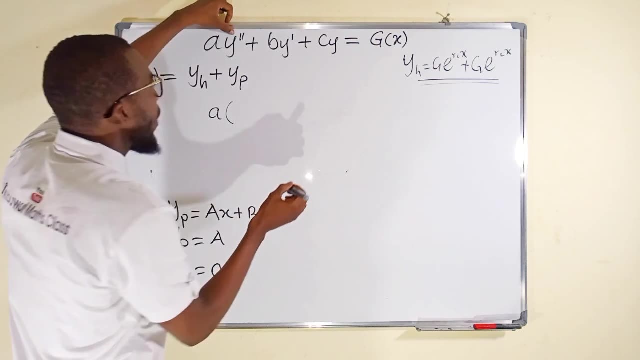 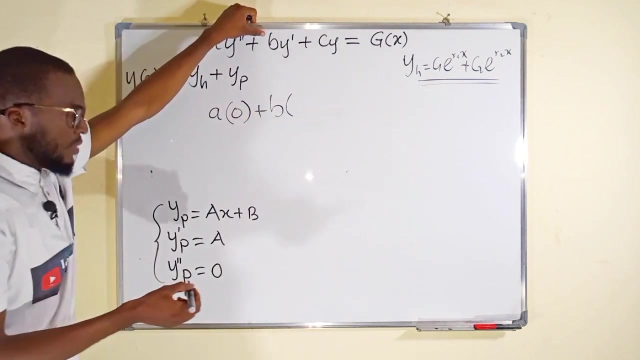 all these three into this general equation. So what we have here is a multiplied by y double prime and y double prime. you can see it is zero here, plus b multiplied by y prime and y prime is a plus c multiplied by y. 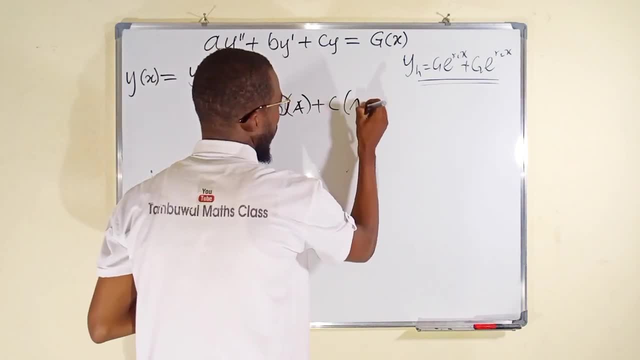 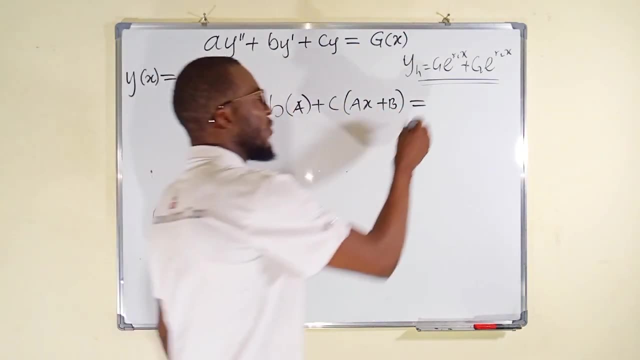 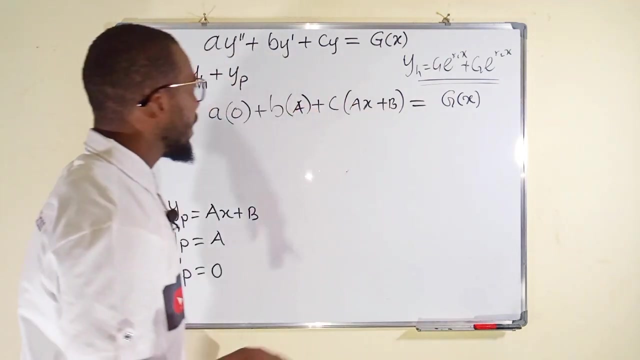 which is the function ax plus b, ax plus b. And remember this must be equal to g of x, g of x, whatever is there. But remember we have set it to be a linear polynomial. So what do we do next? 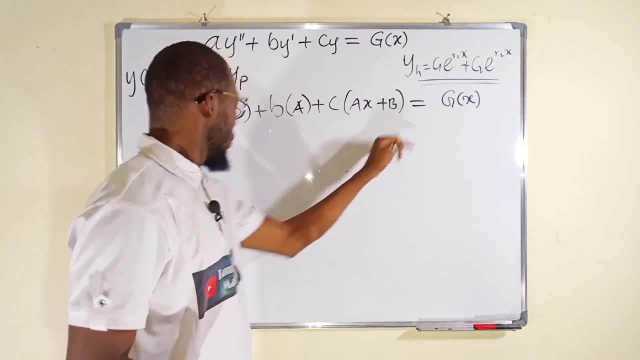 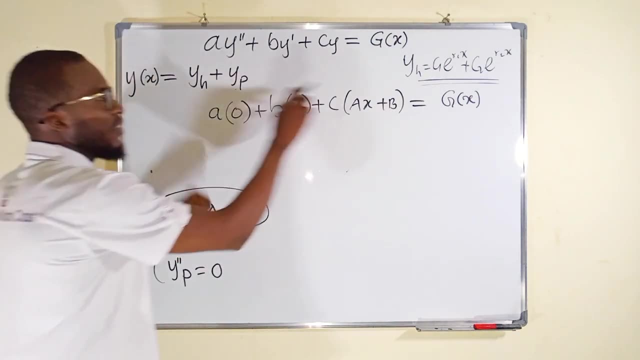 In the end we want to find the values of a and b. Then we replace them back here, which is this: y sub p, and already y sub h is equal to this. So what we have is said to be the solution. 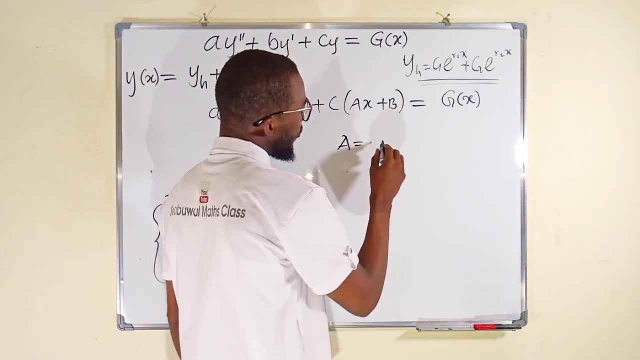 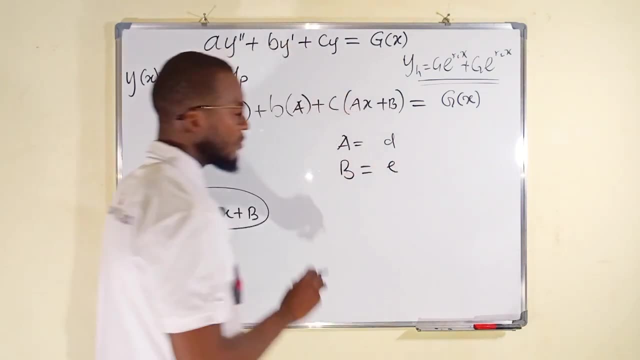 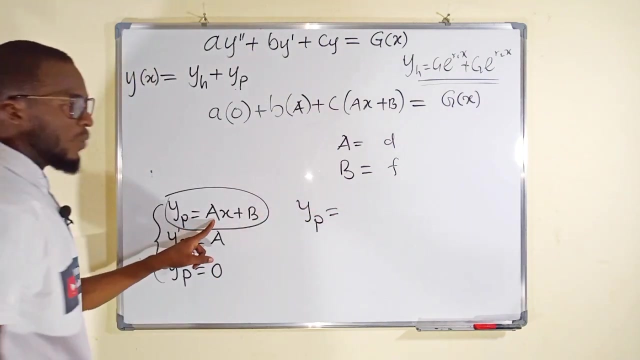 So suppose our a- we have obtained it- to be equal to maybe d and our b to be equal to e or f, let me call it f. So what do we do? y sub p will be equal to a, is d? 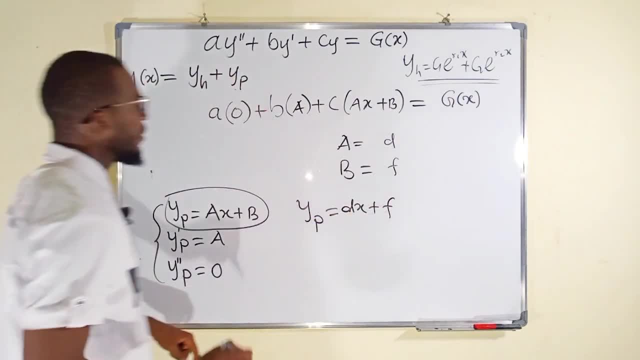 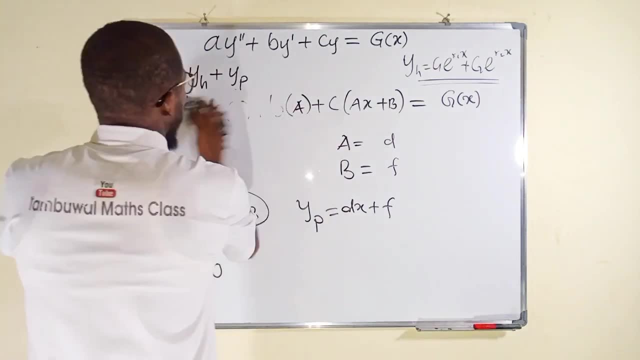 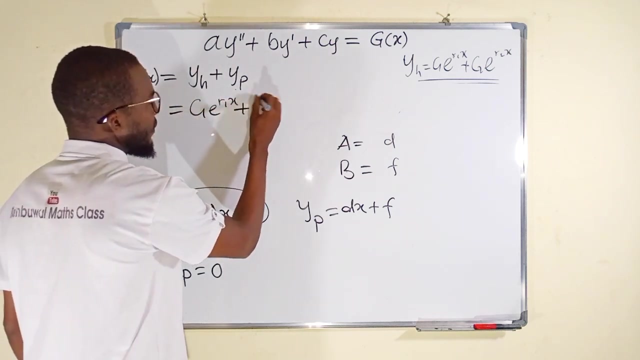 we have dx plus b is equal to f. So the general solution will be equal to y sub h plus y sub p. and let me write it for you: y sub h is this: c1 e to the r1, x plus c2. 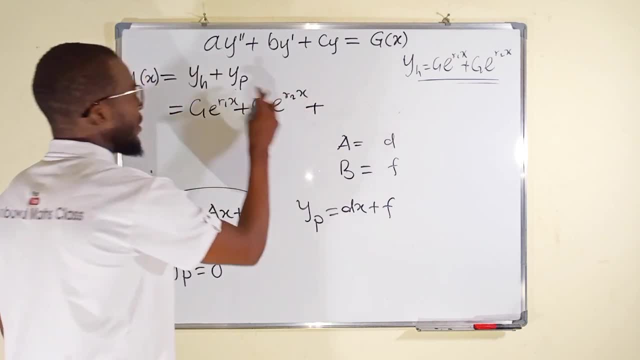 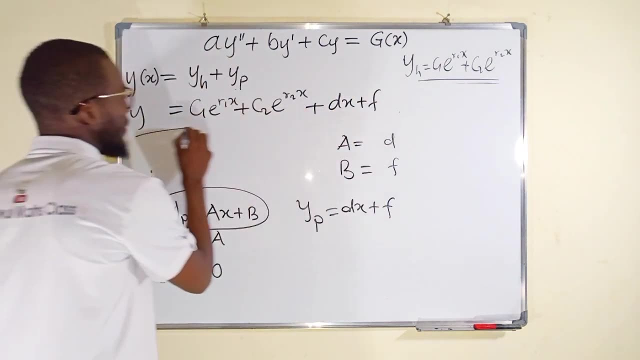 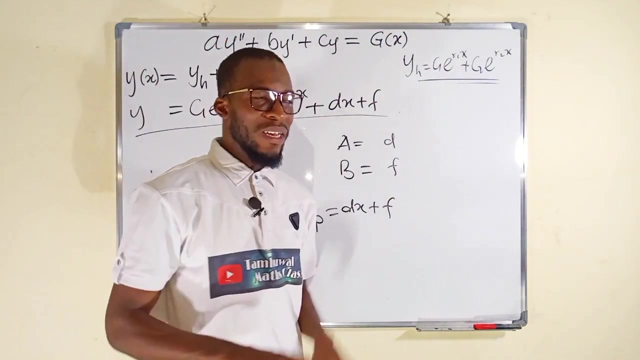 e to the r2 x. Then you add a particular solution, which is dx plus f, So this is y and this is said to be the general solution to this second order linear non-homogeneous differential equation. This is all I have for you today. 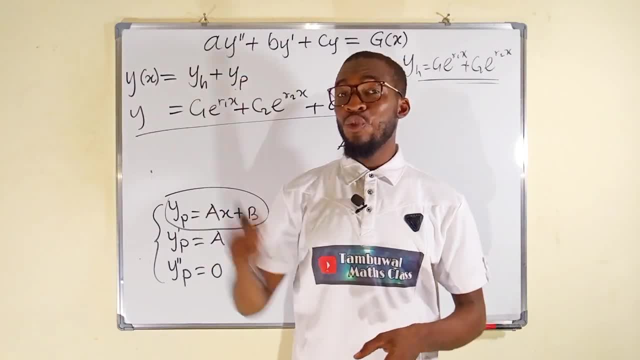 Subsequently, you are going to be dealing with problems under this second order: linear, non-homogeneous differential equations- Bye-bye.